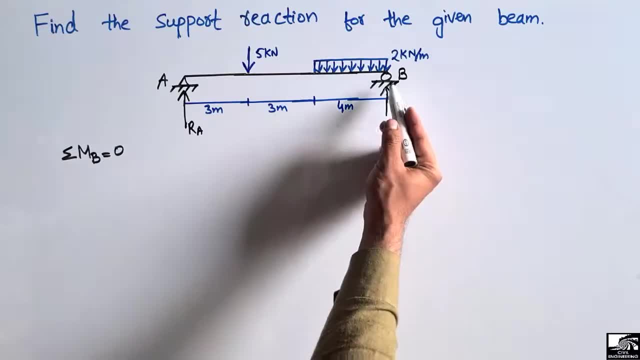 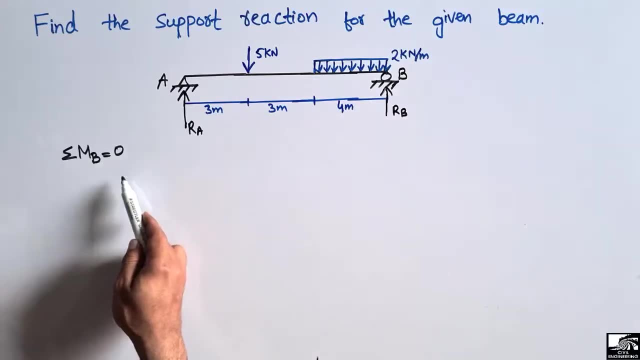 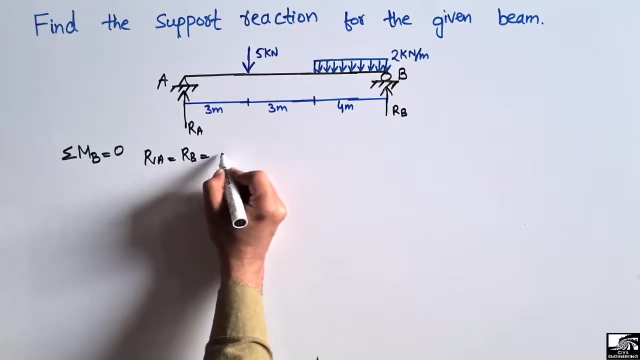 this case we are going to take the summation of moment at point B equal to zero. So we will take all the moment about point B And then we will take the summation of all these movements equal to zero. So we know that RA and RB, these are unknown to us. 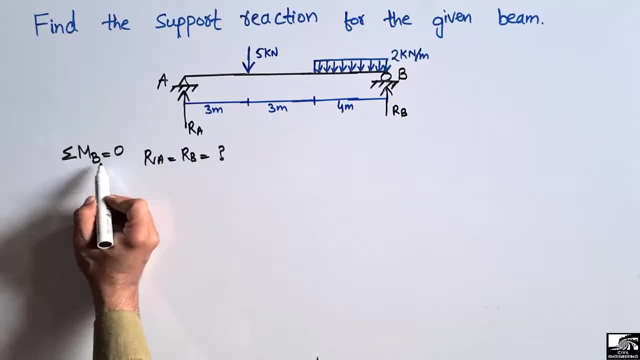 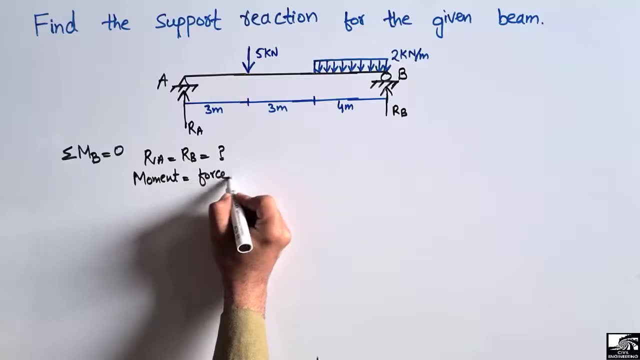 So these are the required data. Now to find out the movement. we know that the movement formula is force multiplying with the moment arm, So we will find the force, and then multiplying with the moment arm, so we will get the moment. 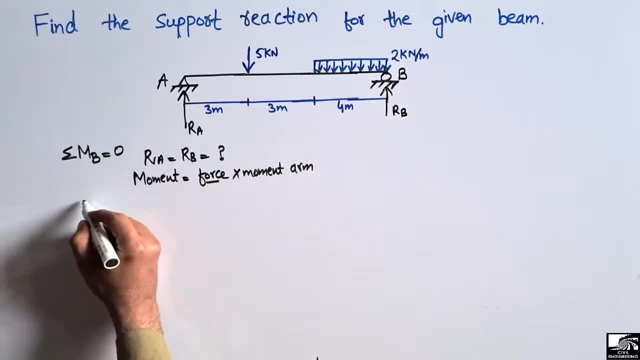 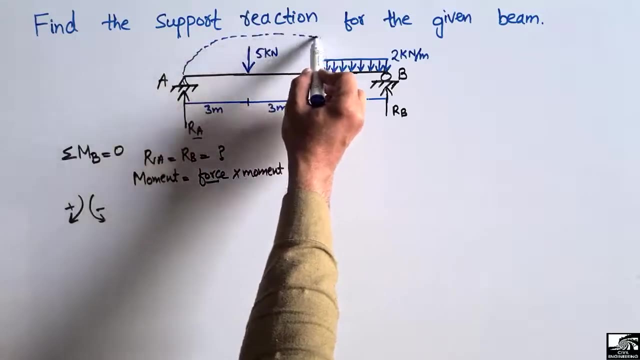 So to find out the summation of movement at point B, let's consider: the clockwise movement are taken as positive and the anticlockwise moments are taken as negative. Now, starting with this RA, it is acting in upward direction and it will create movement in the clockwise direction about point B. 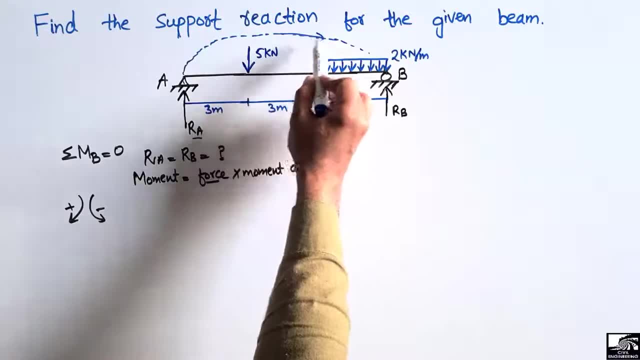 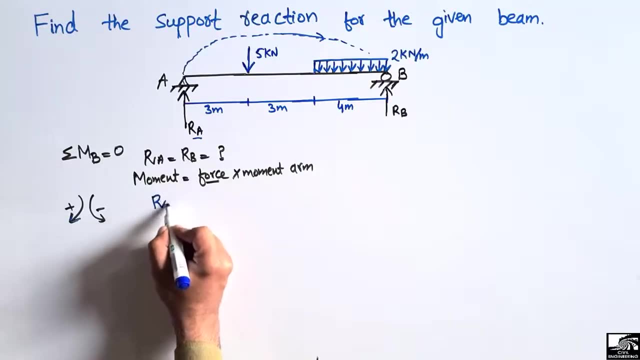 So it will create clockwise movement. So it will create clockwise movement here in this way, which is acting in the clockwise direction about point B. So that's why it will be taken as positive, because clockwise movement are taken as positive here. 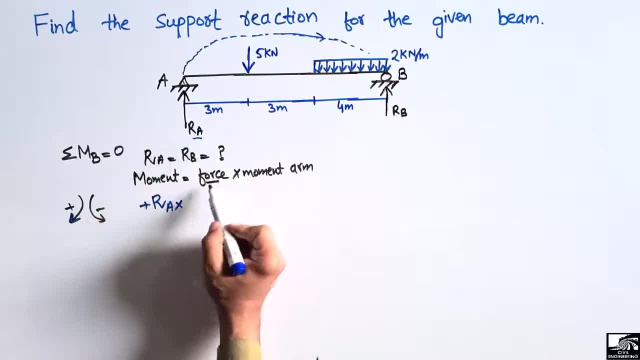 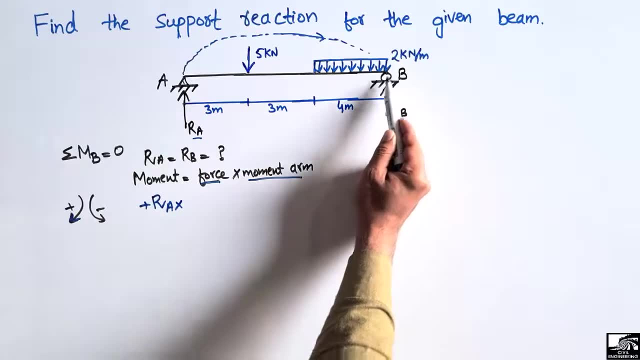 So it will be positive. This is the force. RA is the force multiplying with the moment arm. The moment arm for this force is the distance from this end up to this point, because we want to find the moment at point B, So it will be 3 plus 3 plus 3.. 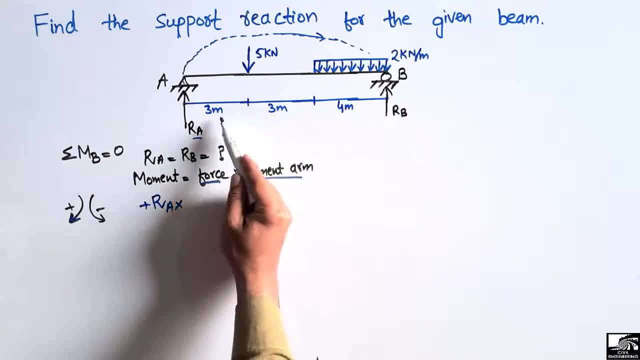 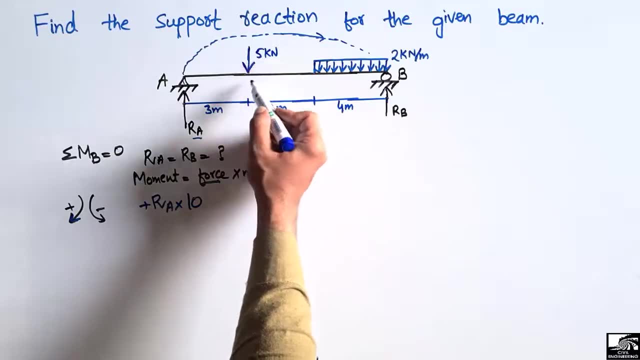 So the total distance will be 11.. 3.. 3., 6 plus 4. This will be 10.. So it will be 10.. And then this force, 5 kilonewton, again creates a movement about point B. 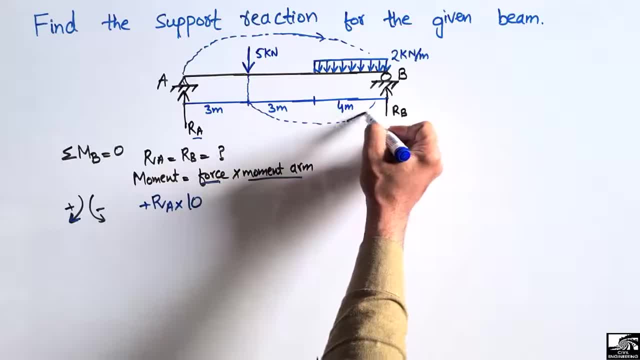 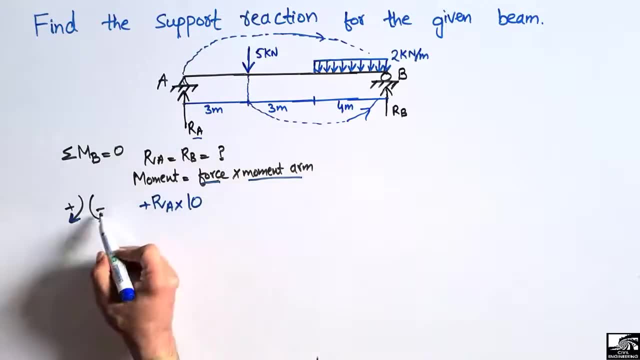 But this moment this will create a movement in the anticlockwise direction about point B because it is acting downward. So it will create anticlockwise movement and anticlockwise movement are taken as negative, So it will be minus 5 multiplying with the moment arm. 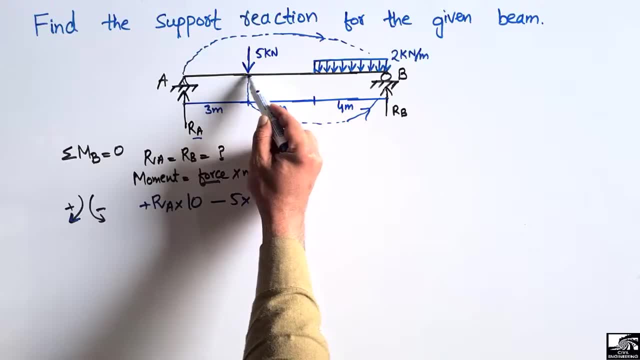 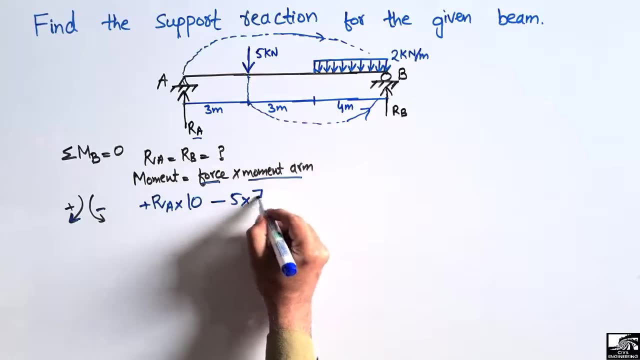 The moment arm is the distance from this point on which the force is acting. So it will be minus 5 to the point B. So it is 3 and 4 which will be 7.. So these are the two moments. 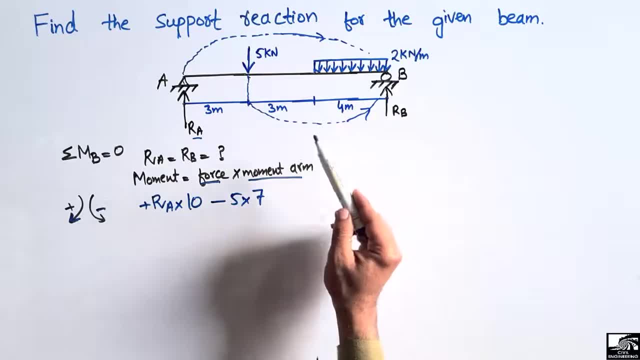 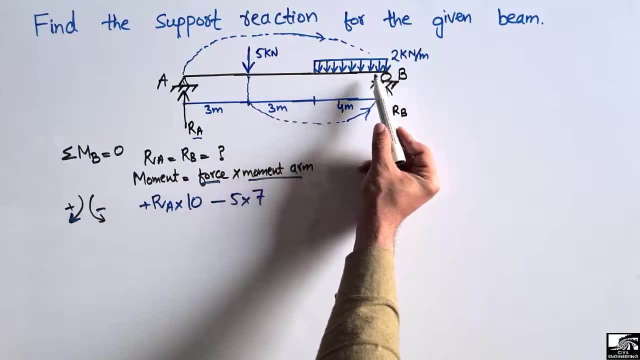 Now, also, this load creates a movement about point B. So how to find out this moment? So this is the distributed load. So first we have to convert into pointed load. So this 2 kilonewton is acting over the distance of 4 meter. 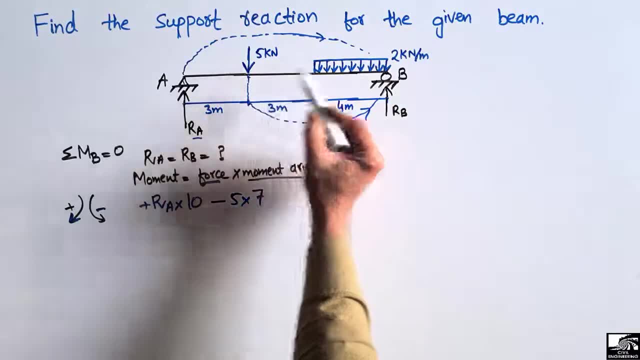 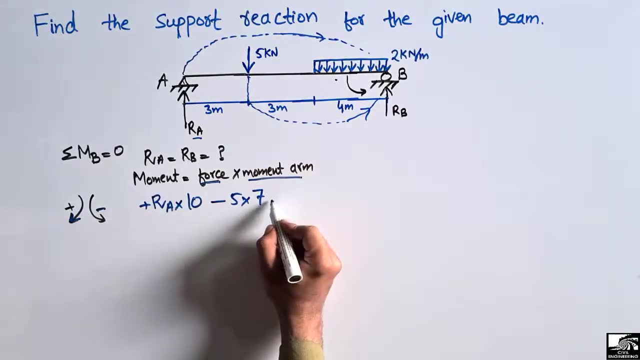 So it will. it is acting downward in the same way as 5 kilonewton, So it will also create the movement. So this is the distributed load. So this is the distributed load And the anticlockwise direction. about point B. 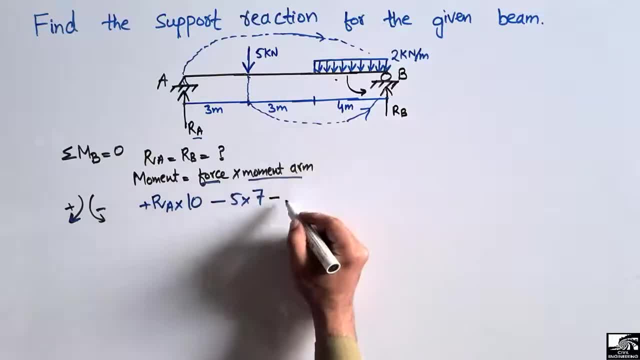 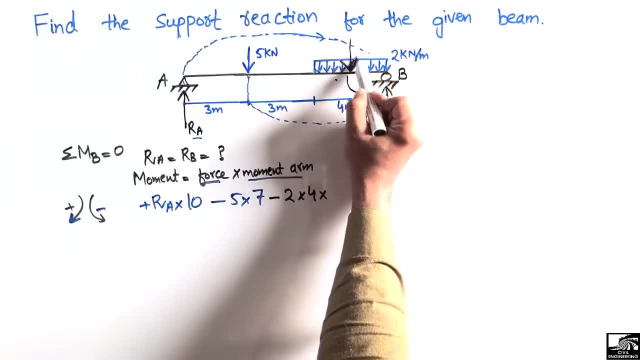 So it will be again taken as negative. Now this is a 2 kilonewton load distributed over the 4 meter, So it will be 2 multiplied with the 4, multiplying with the moment arm. So this force acts at the center of this distributed load. 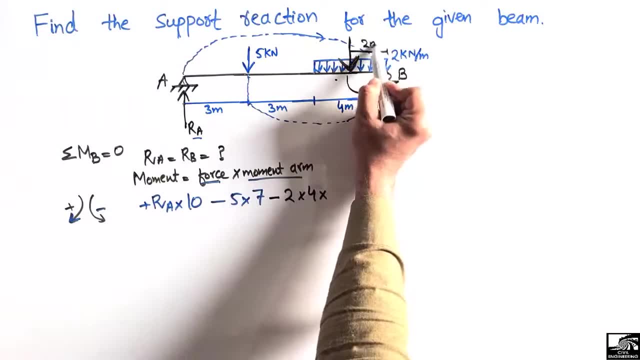 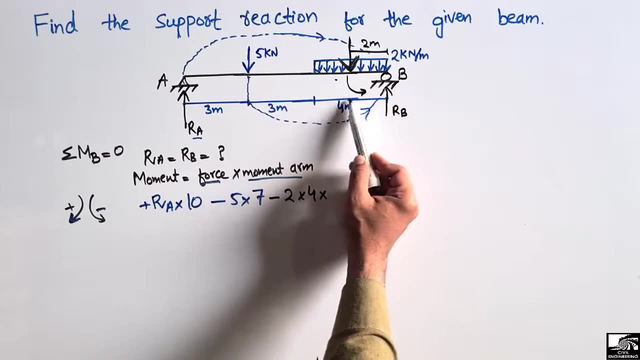 And this at the center of 4 meter. So this moment arm will be 2 meter Because it acts at the center of this uniformly distributed load And this is the distance of 4 meter. So the half of 4 will be 2 meter. 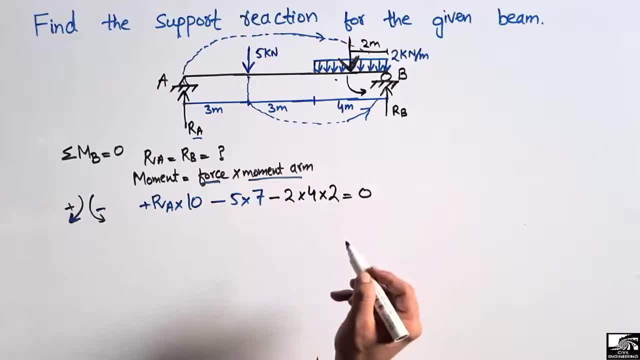 So it will be 2.. Summation of all the moment about point B equal to 0.. Now 10 Ra. If we shift this value into the right side, we got 16 into 35. Now Ra comes out to be 51 dividing by 10.. 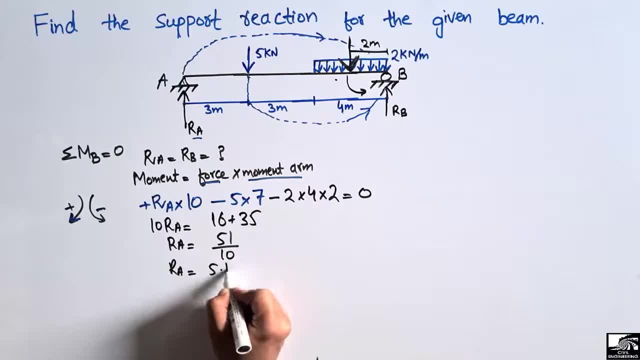 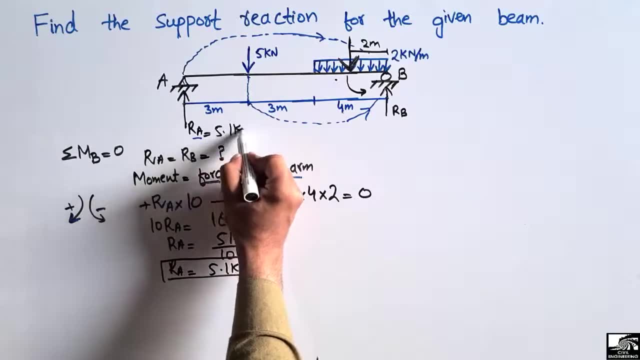 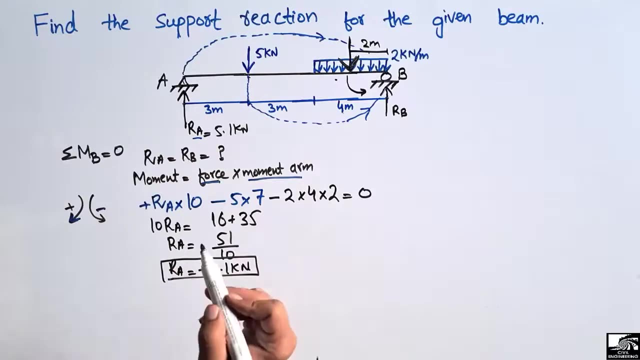 So Ra comes out to be 5.1 kilonewton. Ra comes out to be 5.1 kilonewton, So we assume that it is acting in upward direction. So we have plus sign here. It means that our assumed direction was correctly. 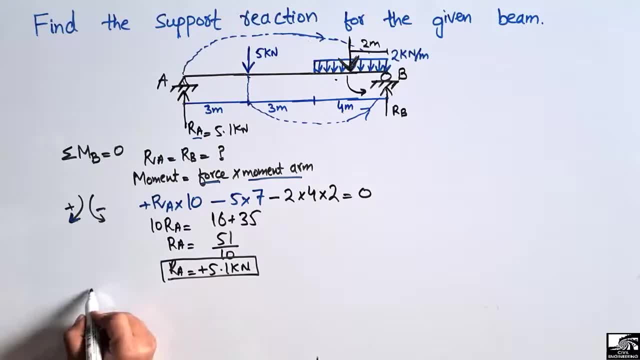 Now how to find out the Rb. So we will take help from this equation, From this equilibrium equation That summation of all vertical forces are equal to 0. And let's suppose the upward forces are taken as positive And the downward forces are taken as negative. 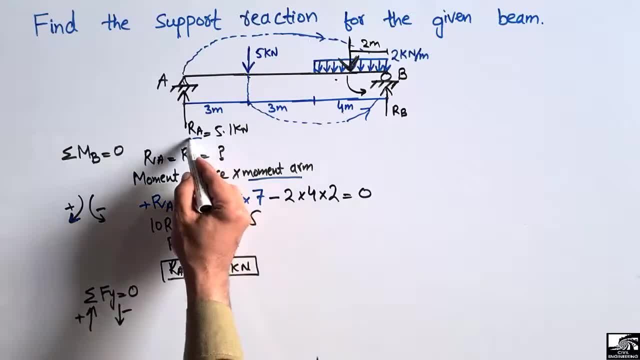 And the downward forces are taken as negative. Now the upward forces are Ra and Rb. Now the upward forces are Ra and Rb. So Ra and Rb, So Ra and Rb. These are acting in upward direction. 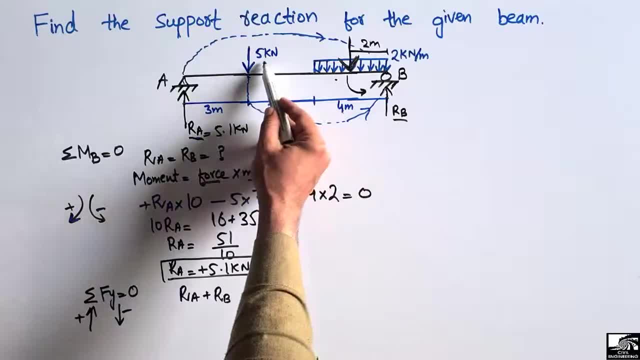 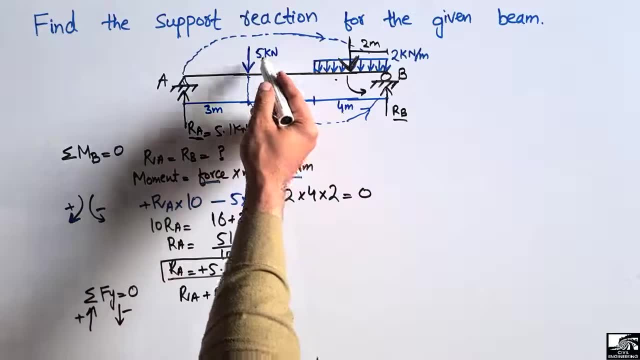 So they are taken as positive. Now this force is acting downward. Now this force is acting downward, So this force is also acting downward. So minus 5 kilonewton. So minus 5 kilonewton. 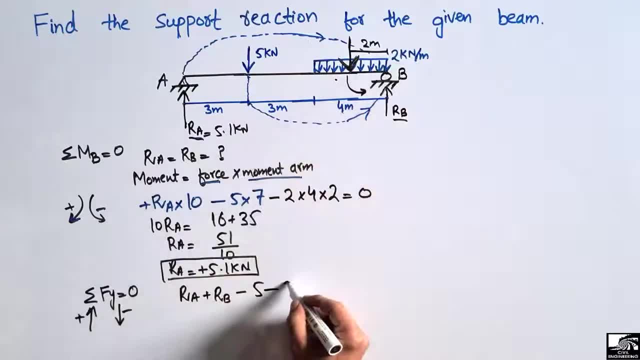 and minus this load which is 2 kilonewton per meter, So it will be 2 multiplied with the 4, because this load is distributed over of 4 meter. So to multiply 4, we have now pointed low. Summation of all the vertical.